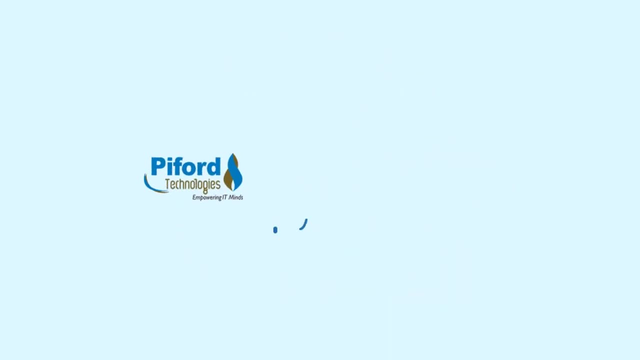 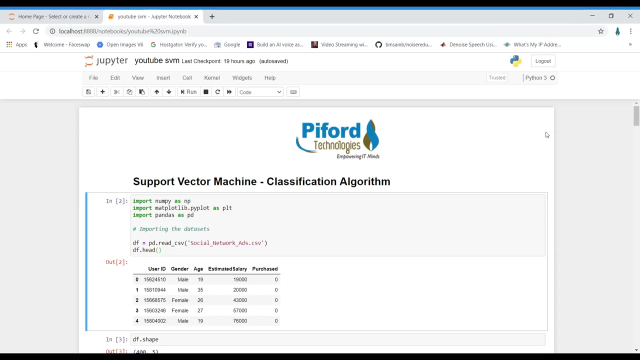 Hi everyone, this side, Arohi from PyFit Technologies, and in my today's video I'll talk about sport vector machine algorithm with practical example. So let's start. So, first of all, I have imported all the required modules, and the data set on which I work upon is 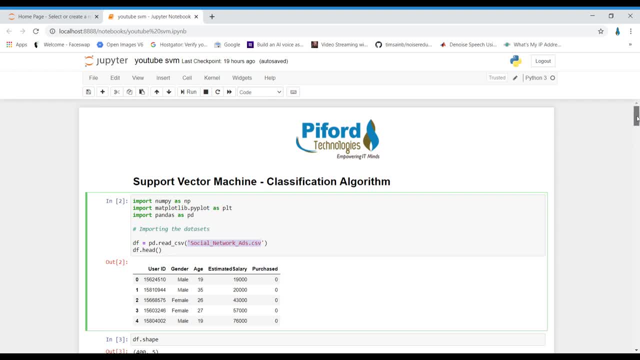 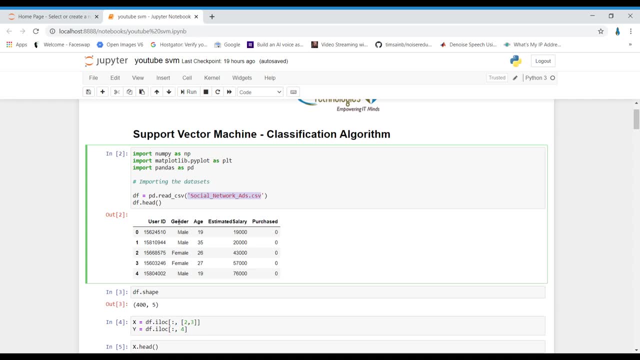 this is the data set, So this is how this data looks like. We have these column, user ID, gender age, estimated salary and purchased means on the basis of gender, age and estimated salary. We want to know, we want to classify, whether person will purchase a product or not. Right, 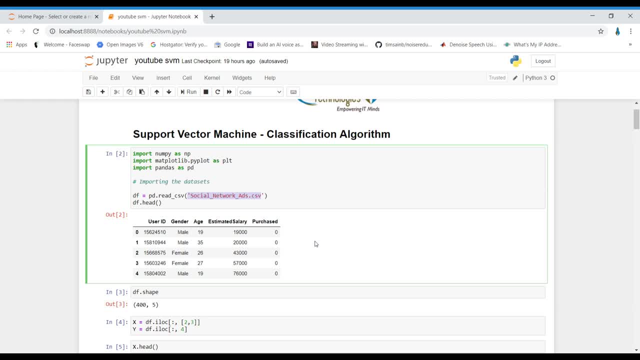 Zero means person will not purchase a product and one means person will purchase a product. So we have two different kind of classes in purchase: zero and one. Zero means not purchased in one means purchased Right. So on the basis of gender, age and estimated salary. 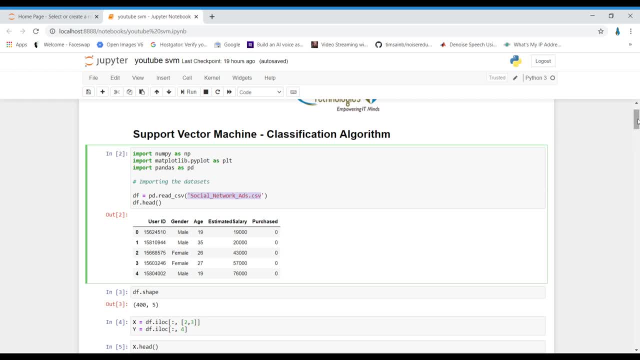 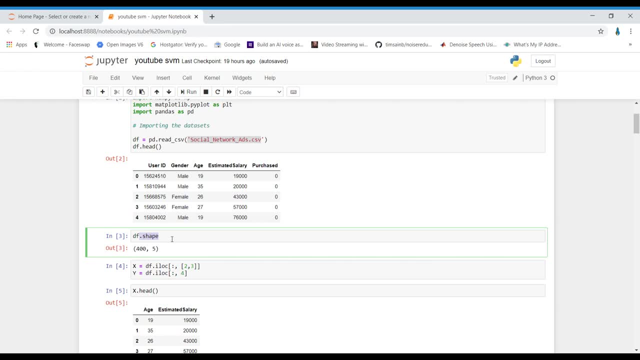 we want to perform this application. So let's see, Let's see some features about data set first of all. So I have checked the shape of data set over here. So we have 400 rows, means we have 400 different records and five columns in this data set. Now let's divide our data set into X and Y. X means independent. 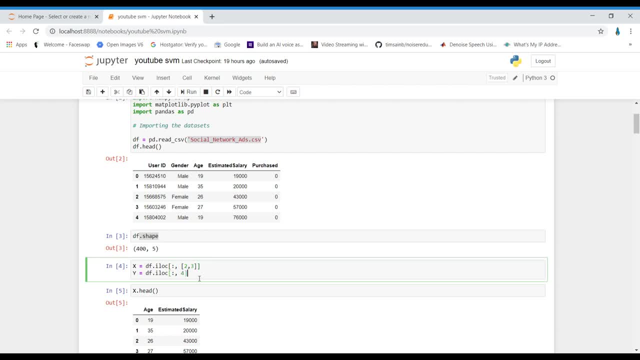 variable and Y means dependent variable. What is Y? What? Y simply means what we want to classify or what we want to predict, And X means on the basis of which we want to predict Y. So X is independent and the Y of value of Y is dependent on X. 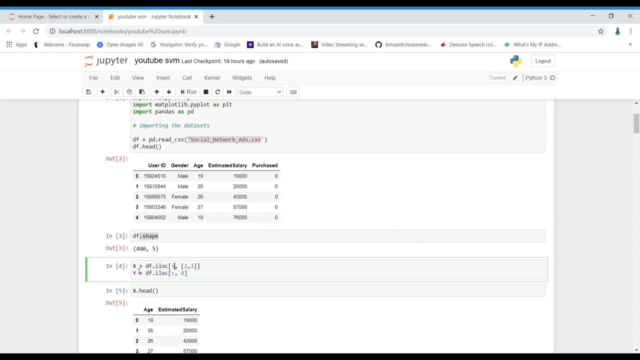 Right. So after seeing X, What all columns I'm using? I'm using second and third column. Second means age and third column is estimated Salary. I'm not using user ID and gender. on the basis of age and estimated salary, I want to see whether person will purchase a product or not. Right. 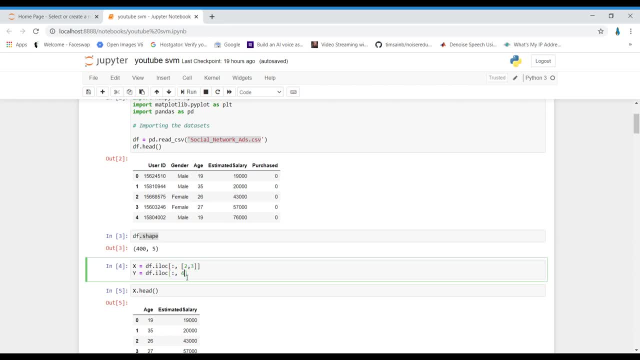 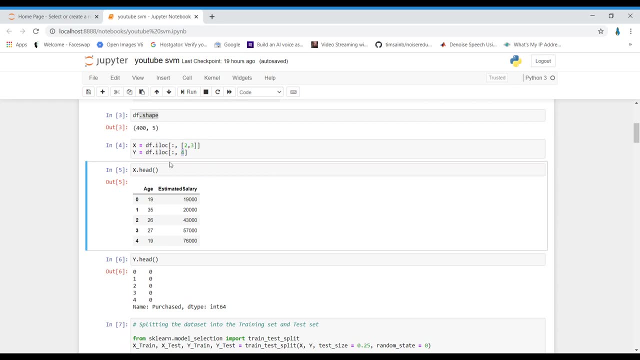 So that's why in X I have two columns and in Y I have column number fourth, which is purchased. So let's print X and Y values separately. So you can see when I print this X value. we have age and estimated salary as a data in X and in Y. 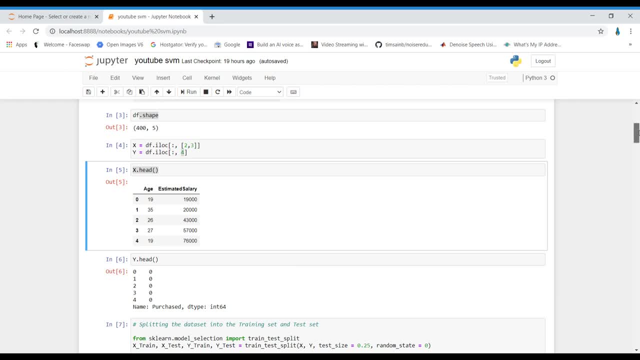 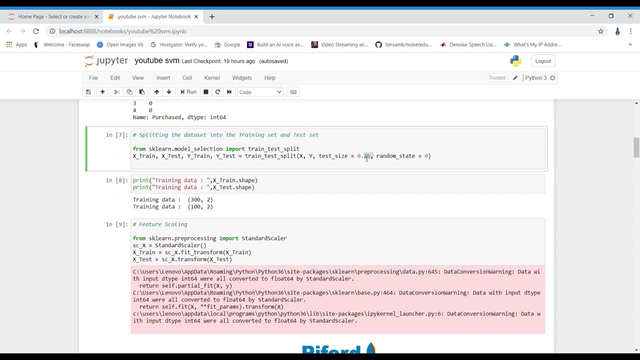 We have Class labels right, So now the next task is to divide your data into train and test. So I'm dividing my data into train and test and test. split is 25% Means remaining data will be used as training data and 25% of data will be used as test data. 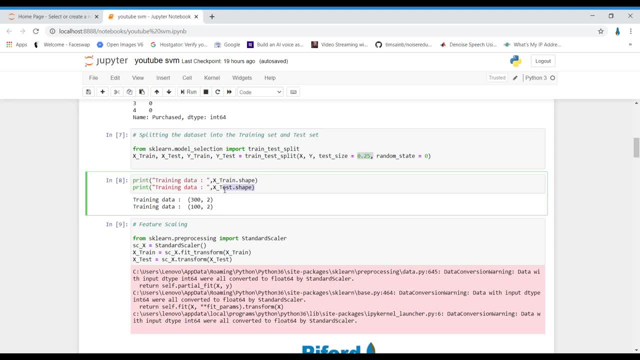 So after dividing my data into train and test, I'm checking the shape of train, X train and X test. So we have 300 records in X train and we have 100 records in two columns in test. data means on the basis of 300 records. 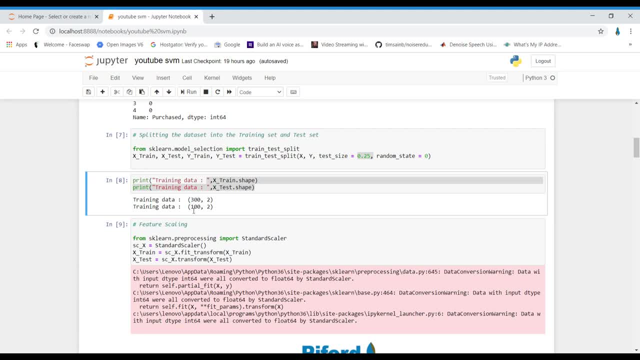 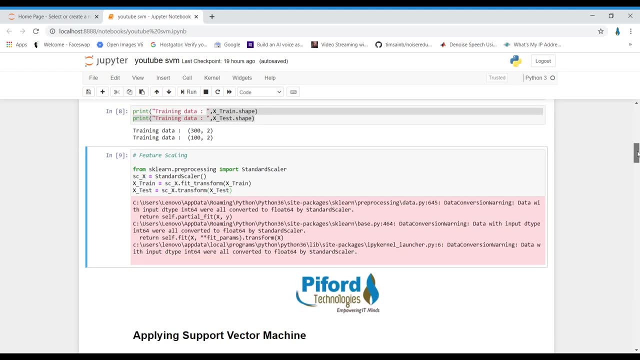 We want to train our algorithm and and after training we will test our algorithm on these hundred records, right? So in next line, in this cell, I'm performing, I'm doing some scaling on the data by using standard scalar. You can even use minmax scalar, but over here, 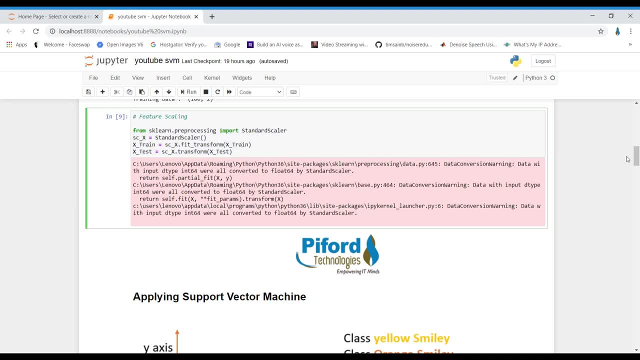 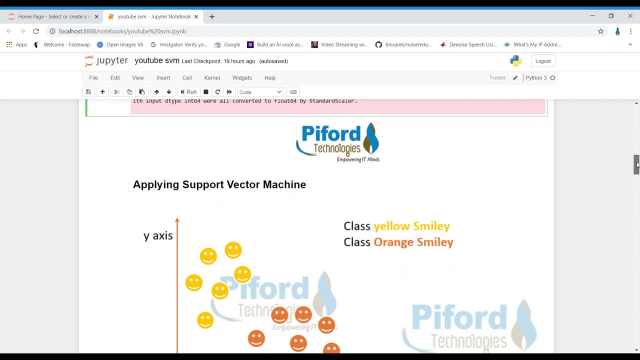 I'm using standard scalar to scale the data right. So after scaling, Now the task is to apply support vector machine algorithm for classification. So first of all, let's understand how SVM classify right, How SVM perform classification. So basically, the job of SVM is to perform classification by finding the right hyperplane that classify the data points in a best image. 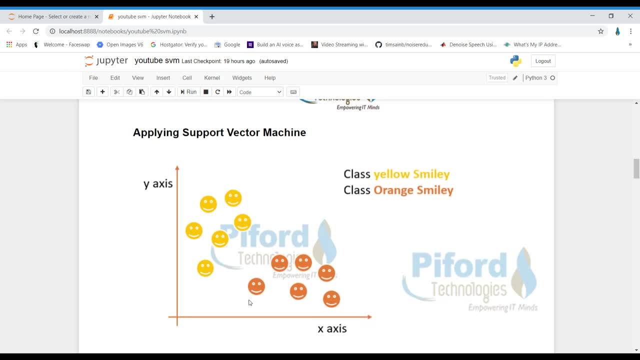 Let's see this image. Suppose we have this data set: Orange smileys and yellow smileys- These are the two different classes, right? And we have data set looks like this: Now we want to perform classification on this data And, as I've told you, SVM perform classification by, you know, by finding a right hyperplane. 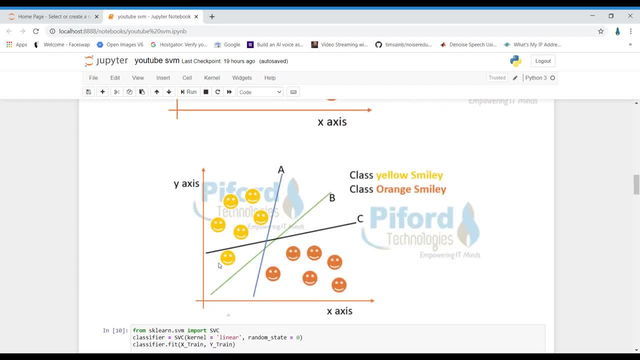 So what is that hyperplane? Let's understand this. See on their data. I have three hyperplanes: One is blue hyperplane, One is green hyperplane and other one is black hyperplane. So this blue hyperplane, Let's talk about this hyperplane. 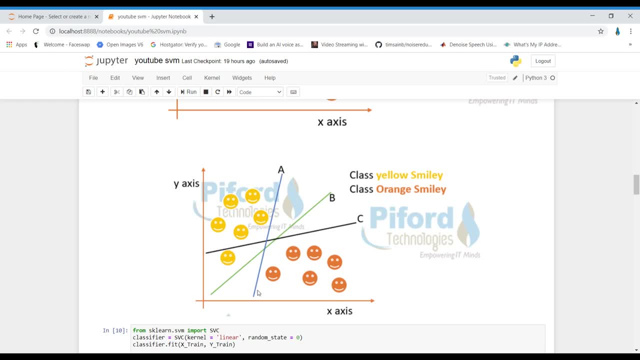 First of all. so if you'll see this hyperplane, so what we can say is: see over here that this data point is very close to this blue hyperplane means the gap between this data point and line is very small. On the other hand, if we say orange smileys over here, this orange smiley is also very close to this blue data point means classification is being done properly. 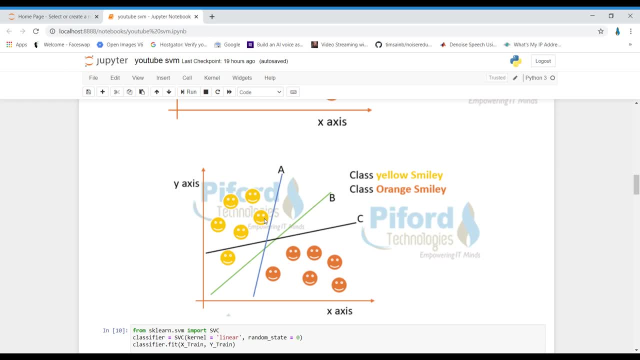 But the thing is distance, the gap between the closest data point and the line and the gap between here. Also, the gap between orange smiley and this blue line is very small. right, And how we choose right hyperplane over here We have three hyperplanes, right. 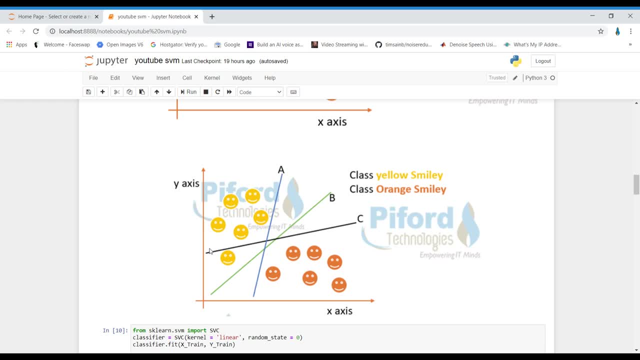 So if we talk about this black hyperplane, so this black hyperplane will not be acceptable over here because this is performing misclassification. We are not, even the data Is not getting classified properly, So will not choose this black hyperplane Now. 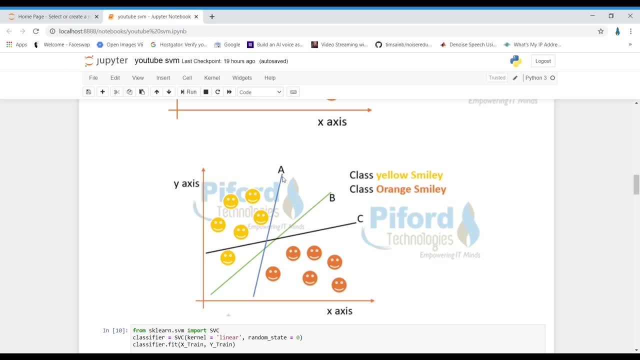 The thing is how to choose, like, between this blue and green hyperplane, which one is the best hyperplane, How to choose that? So we simply choose the line, We simply choose the hyperplane with the maximum distance from the closest support vector. 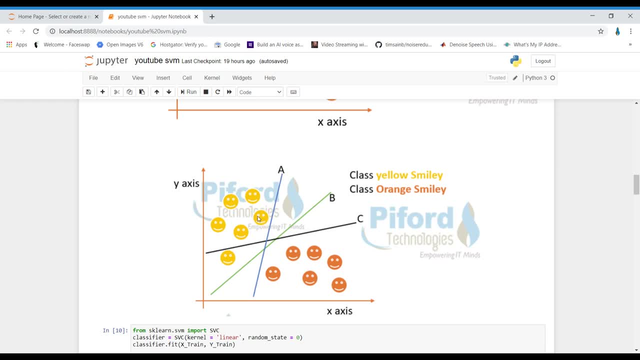 See support with this data point. The closest data points are also Called support vectors. You can say it closes data point also and you can say it support vector also. So how will choose the right hyperplane by the will see that the maximum, the line which have maximum distance from the closest support vector. 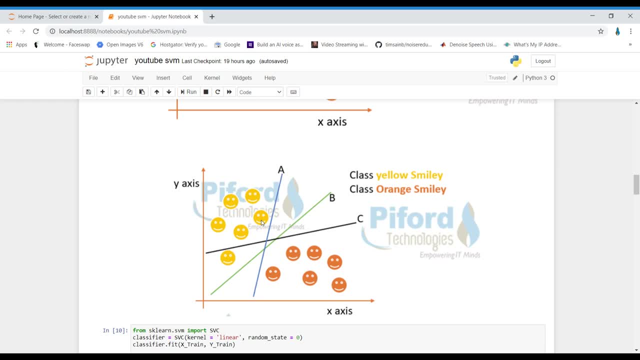 So, out of these three lines, out of these three hyperplanes, we can see that the green hyperplane has maximum distance from the nearest support Vector, maximum distance. So which yellow smiley data point is closest to this green vector, green line? this one. 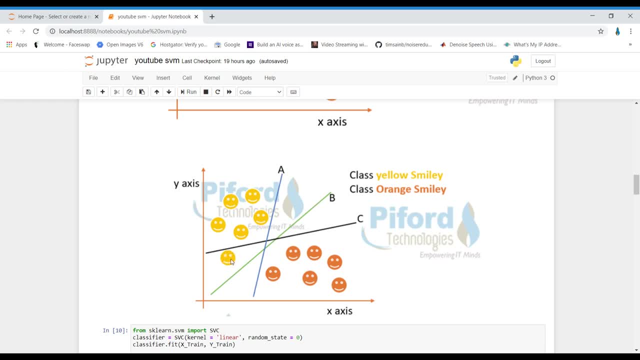 So this is the closest support vector to this green hyperplane and this orange data point is orange support vector is closest to this green hyperplane. Now, what we are checking over here is the hyperplane which has maximum distance From the nearest support vector. 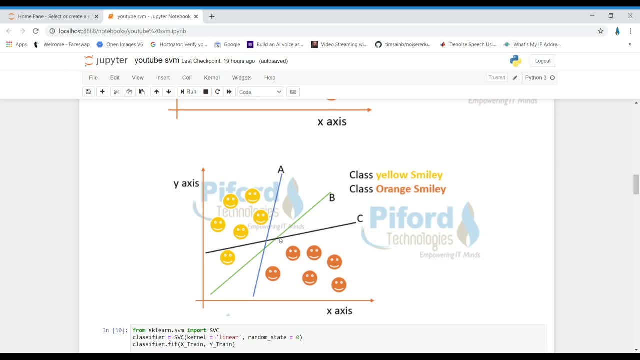 So, out of these three line, green line is the line which has maximum distance from the closest support vector, So we'll be choosing green hyperplane as the right hyperplane. So this is how SVM work. Now let me show you, with the coding, how to execute this whole thing. 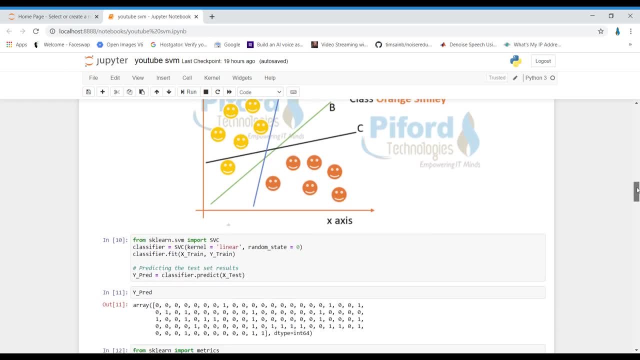 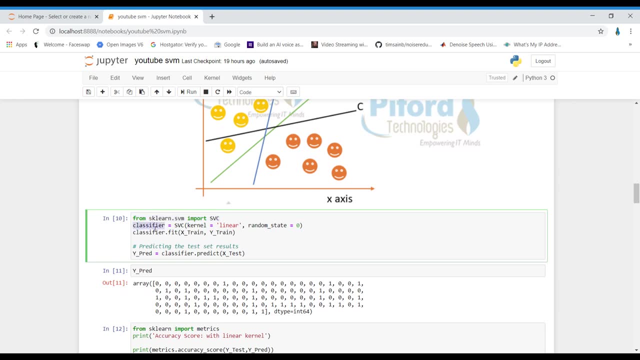 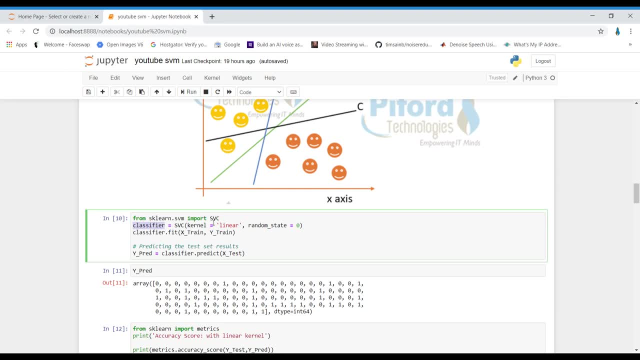 So classifier is a variable in this variable. I'm calling this SVC support vector, SVC module- Sorry, algorithm and the kernel I'm using over here is linear. see in SVM, in support vector machine We have a various different kernels, right? So SVM is famous for its kernel recalling. 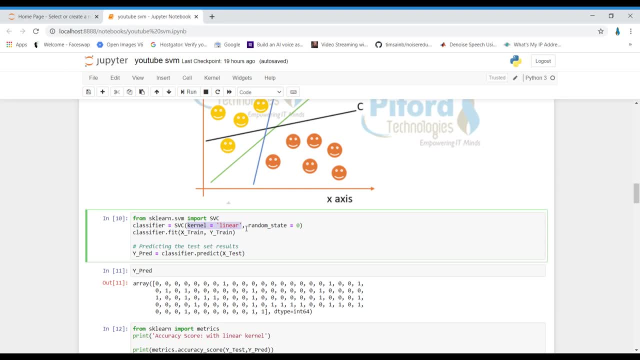 So we have various kernels like linear kernel, RBF kernel, polynomial kernel And sigmoid kernel, right? So I'll be using two, three kernels over here just to show you how different kernels will give you different results. The very first kernel is linear kernel. 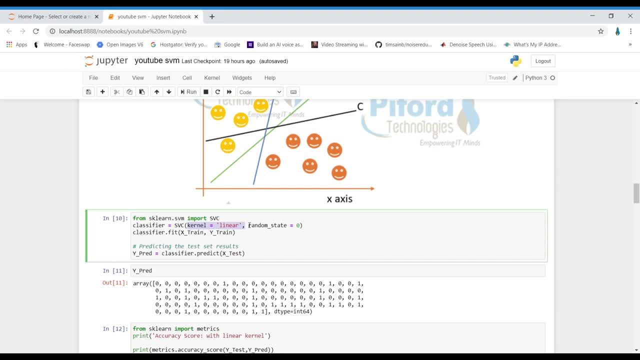 So I'm a kernel, I'm using is linear kernel, and then I'm training my algorithm. So we all know like, by using this fit method, We can train our algorithm by giving it X train and Y train data right, And then we perform prediction and we perform prediction. 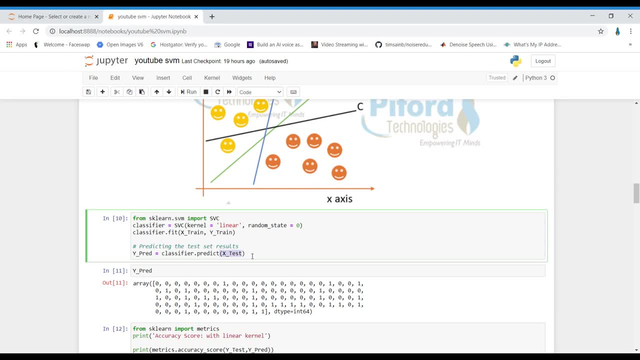 We perform prediction on X test. So how many records for how many records? we have for test data 100 records. So that means over here will be getting 100 different Y values for 100 different X values. right Now let's check the accuracy for SVM algorithm when kernel is linear kernel. 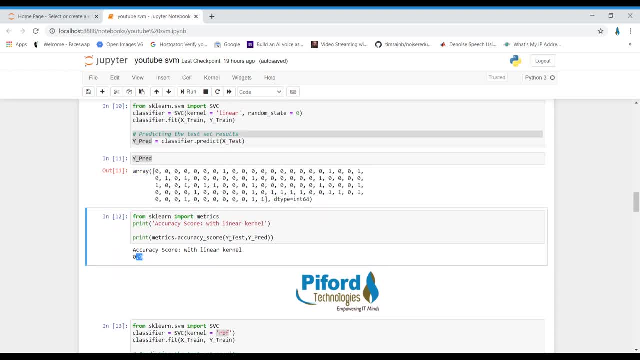 So the accuracy is 90%. So how we check the accuracy? See, We simply check the difference between the actual Y value- Our actual Y value is present in Y test and Y underscore. predict is our predicted Y value. We check the difference between actual value of Y and the predicted value of Y. 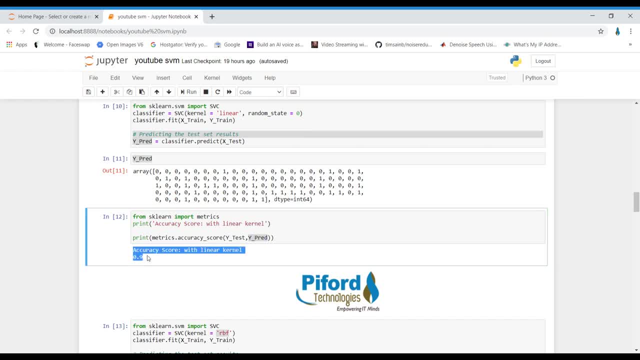 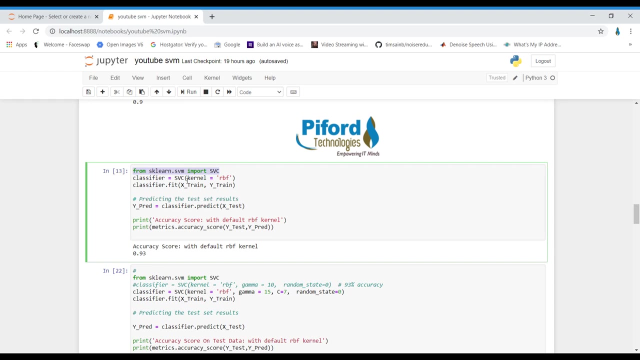 And what we are getting over here is we are getting that our algorithm is 90% correct when we are using linear kernel. Now let's change the kernel and see the accuracy again. So over here again: I'm using the SVM algorithm only. 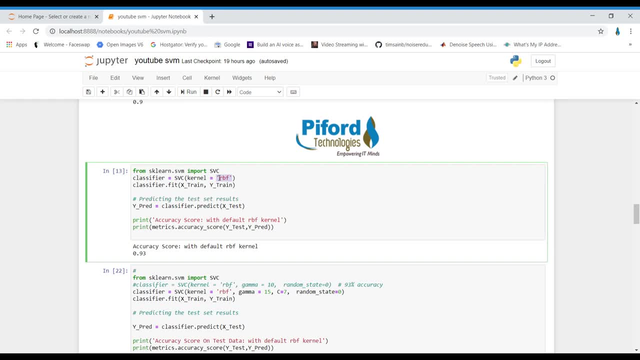 But this time I'm using kernel RBF, radial basis function. I'm using this kernel, So again, fit the data for training your algorithm and then use predict to get the prediction value and then check the accuracy. This time we are getting accuracy 93%. 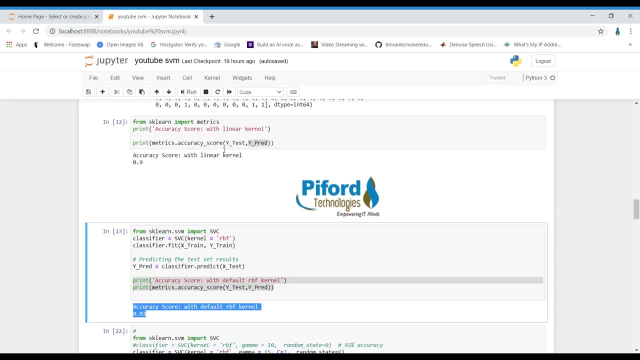 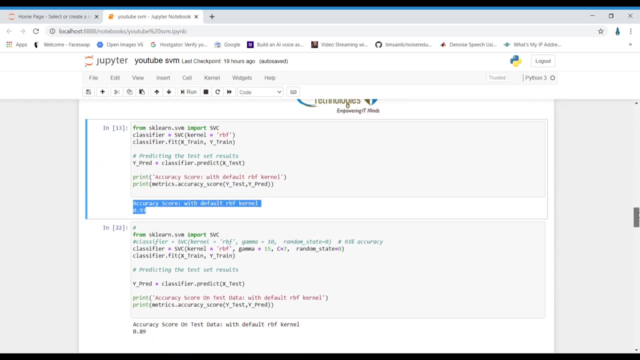 So you can see here that when we have used the linear kernel, at that time we were getting 90% accuracy, But with RBF kernel we were getting 93% accuracy. So now there are other terms. See in RBF when I talk about RBF. 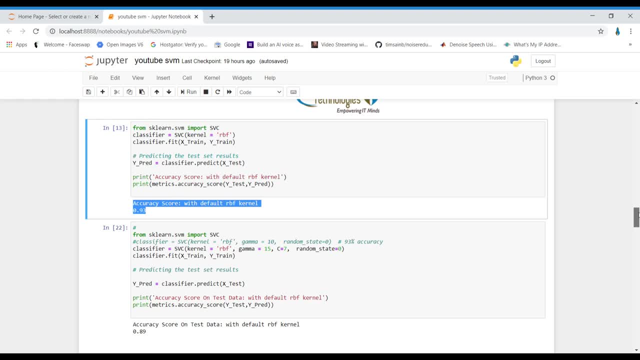 So RBF have some other features also, like we can give the value of gamma, We can give the value of C or term right. So again over here I'm using kernel RBF, But this time I mean you giving other values. 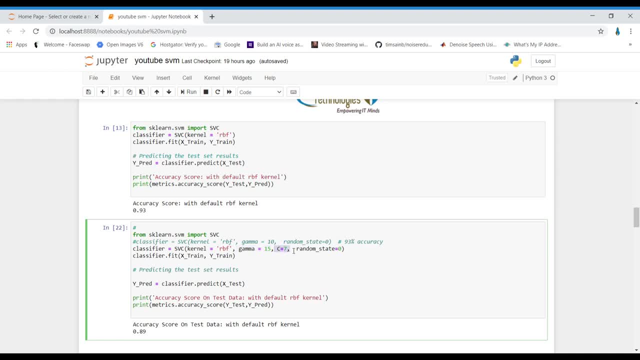 Also, I'm giving value of gamma and I'm giving value of C, right? So when I'm giving value of gamma is 15 and the value of C is 7, at the time I was getting accuracy 89%. See now over here by using RBF kernel. 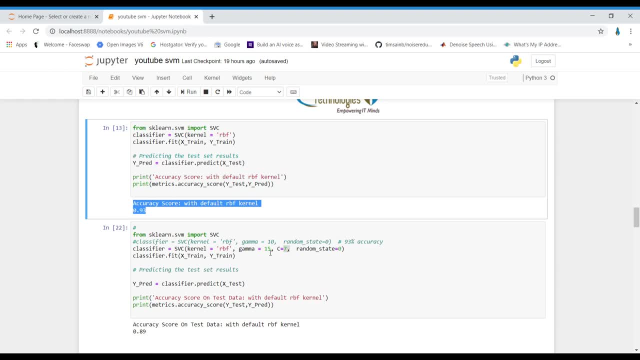 we were getting 93% accuracy, But with the value of gamma as 15 and the value of C as 7, when we use these two values, our accuracy decreased to 89%. So let me tell you what is this? gamma and C? first of all, 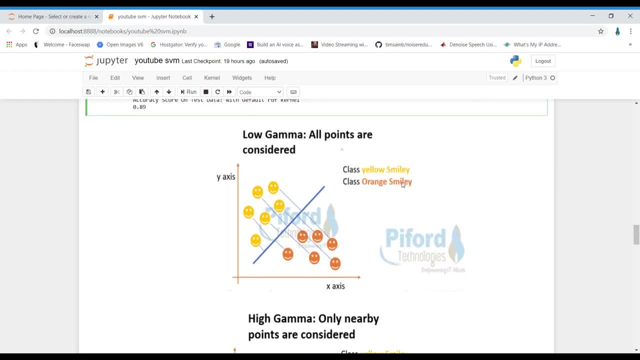 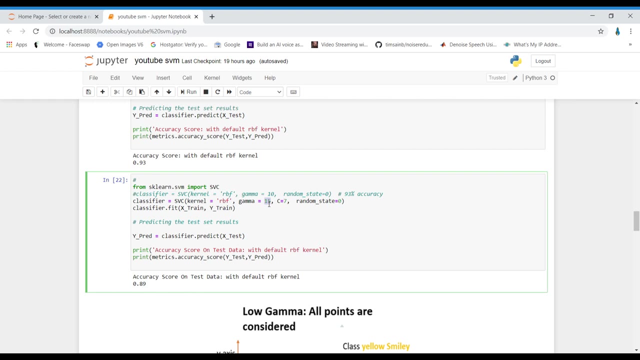 So see, gamma simply means you can see this picture. Gamma simply means if you'll give low value of gamma means if you'll give low value of gamma means, let's suppose, if you're giving one or two or three value of gamma, you assign here three or two or one. 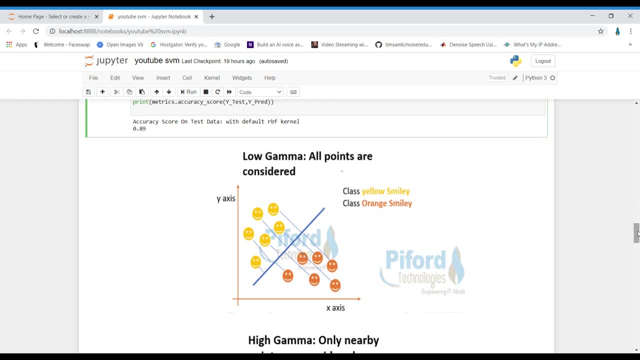 So if you're giving low value of gamma, that simply means for choosing this right hyper plane, we want to calculate the gap between every data point with this line. Right means we'll check what is the. how much gap is there between this data point in this line? 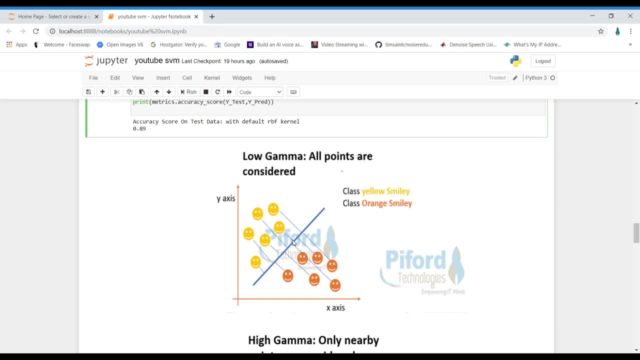 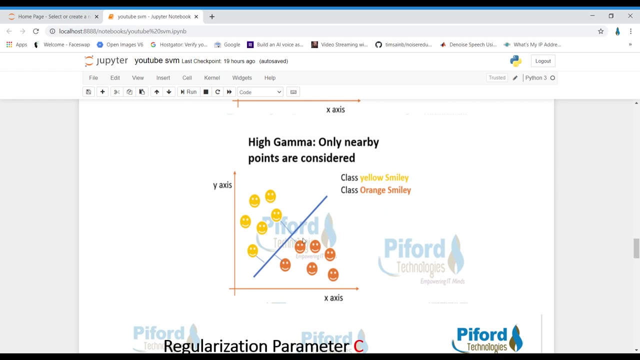 How much gap is there for this data point in this line means, for each and every data point will check the gap between line and the data point. If you're giving low value of gamma And if you're giving high value of gamma, that simply means we want to check the gap between the closest data points with this line. 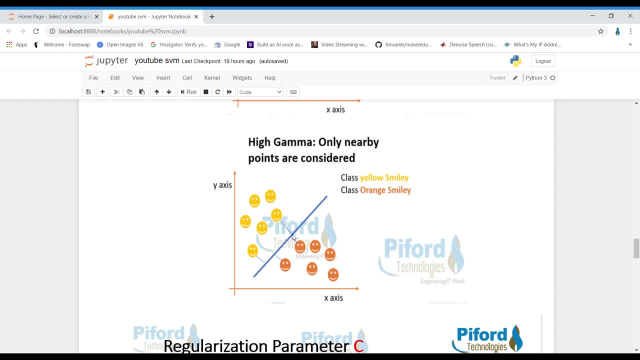 So over here you can see, I'm checking gap between only this with this point and with this point, And on this side also checking gap between this data point in this data point with this line. I'm not calling, I'm not doing it with all the data points. 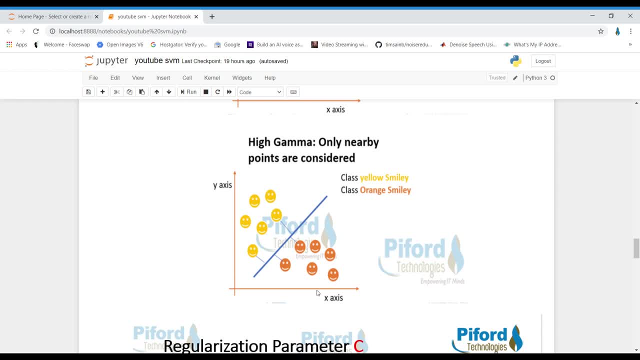 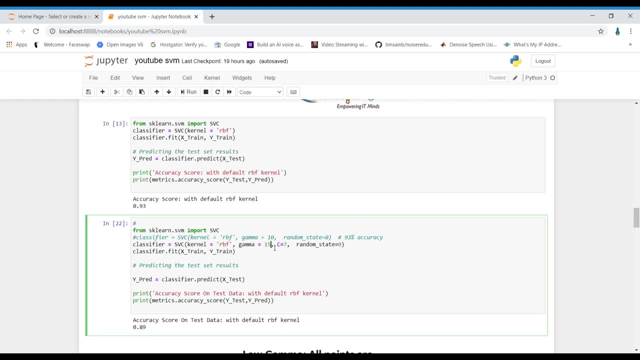 Why? Because over here we have chosen high value of gamma, So that simply means over here the value of gamma is high, Even sorry. What you can do? you can increase or decrease the value of gamma and then you can check the accuracy. 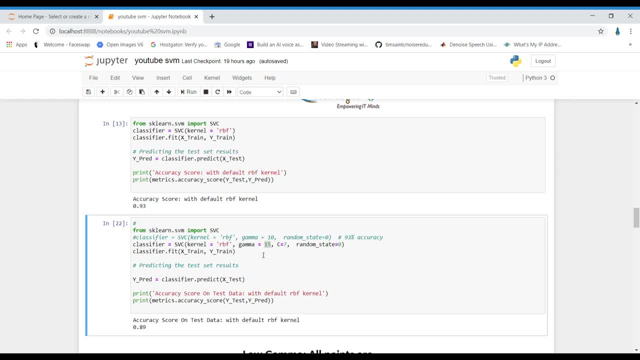 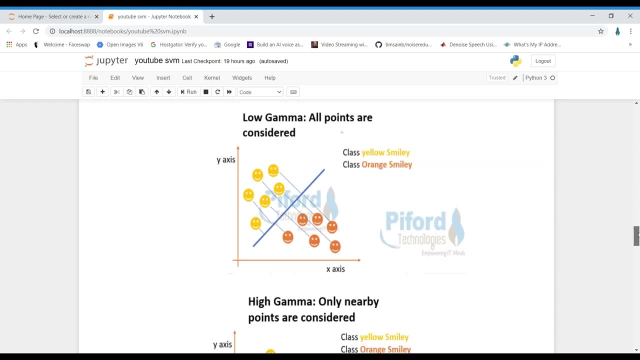 Your accuracy will fluctuate them right in the same way. We have this C over here. The value of C is seven. Now let me tell you how to choose the value of C. So, basically, C is a regularization term. Now what is regularization? 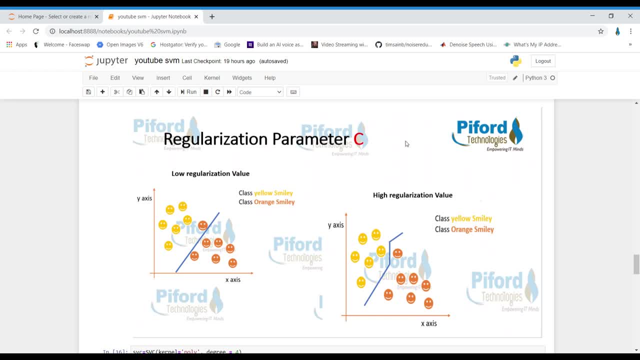 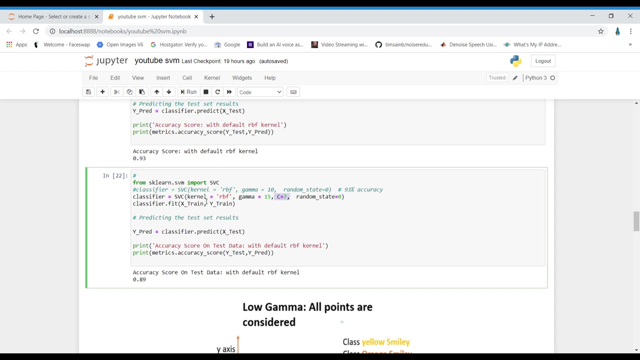 First of all. so regularization means adding some value in the error function to improve the results. So what we are doing over here, We are adding some value right in the error function to improve the results. Now, in simple words, we can simply say that we are using this C term. 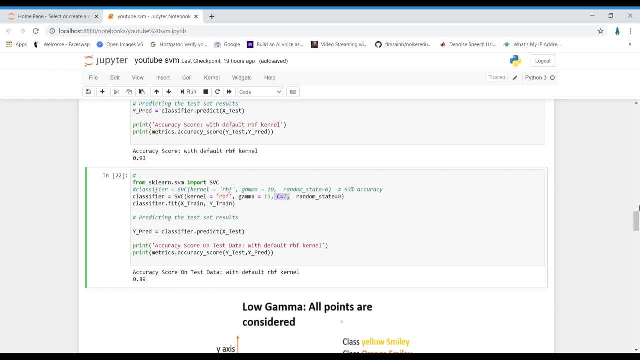 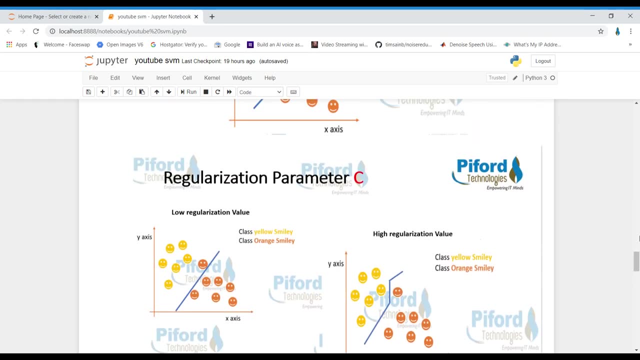 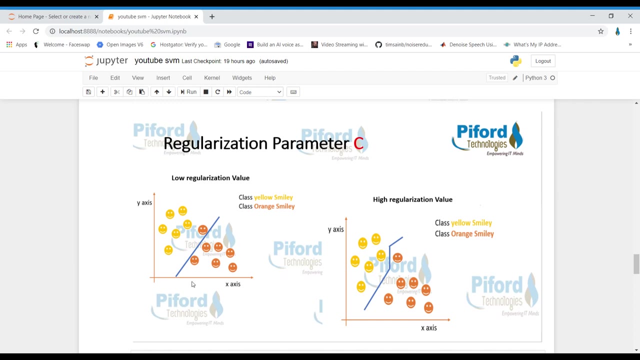 To tell our SVM algorithm how much misclassification to avoid. So if you see this picture, This, these two, this image in this image, these two images are related to this C term. So what if what we are doing in this figure? So if you're choosing low value of C, means if you are choosing C equals to one or two. 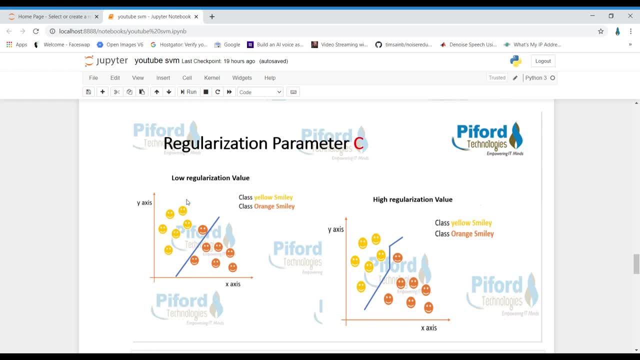 if you're choosing low value of C, then what will happen? See over here. you'll see that when we, when I, have chosen the low value of C, So we are having some misclassification error. So this orange data point should be on this side. 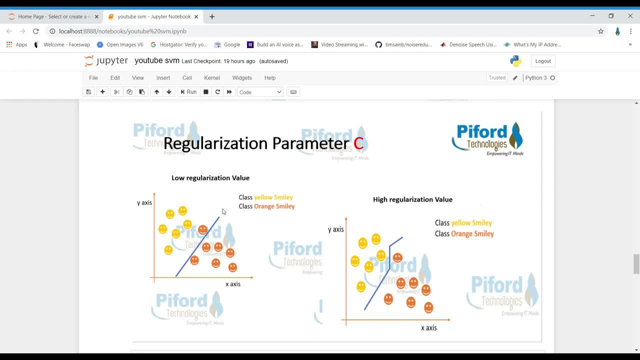 but it is classified as on this side. Why does it happen? Because we have low value of C, So in this side we have higher value of C. Higher value of C means you will get more accurate results. You can see over here. 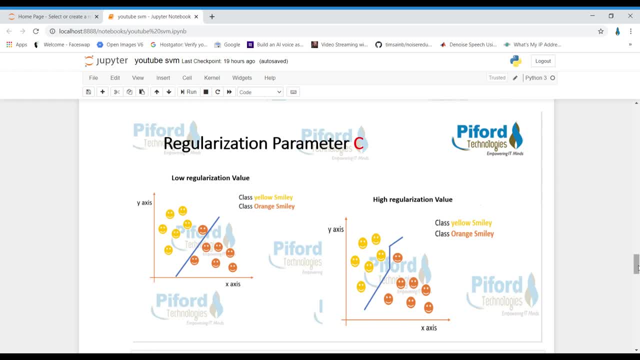 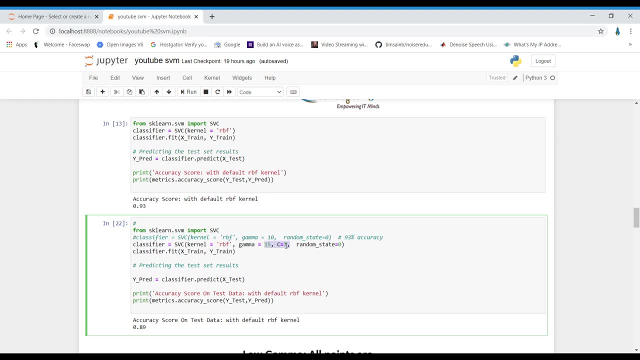 The classification is accurate over here, So that simply means you can choose. There is no any strict rule that like what should be the value of gamma and what should be the value of C, You can choose it yourself. You should only know that what will happen if you choose low value of gamma? 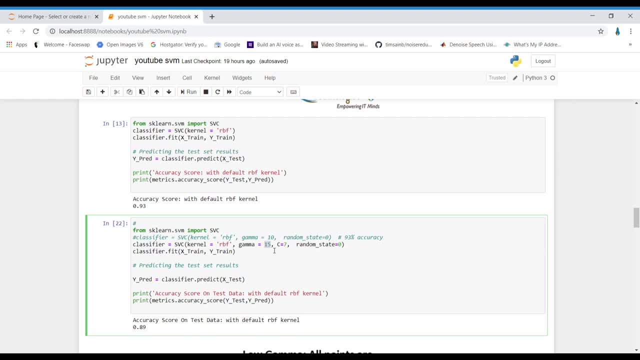 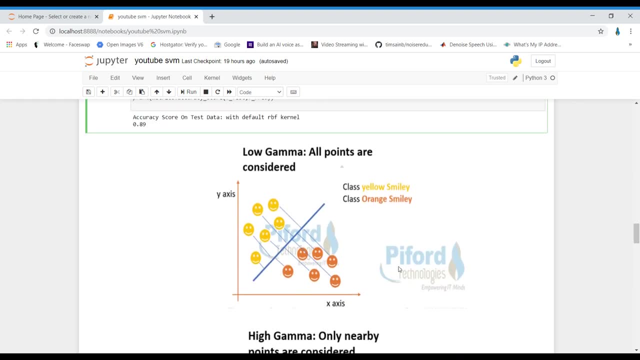 and what will happen if you choose high value of gamma and what will happen when you choose low or high value of C. So that have already explained you. Low value means: consider all points for gamma. High gamma means for this line, choosing this line. 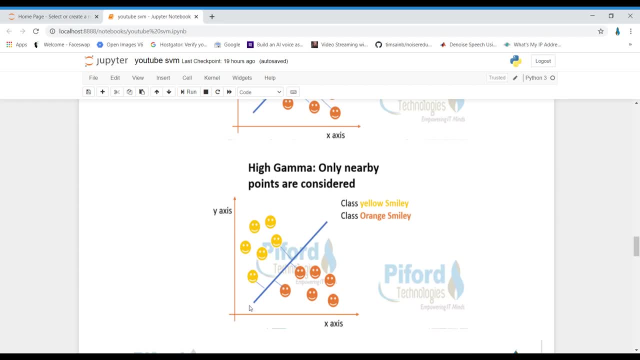 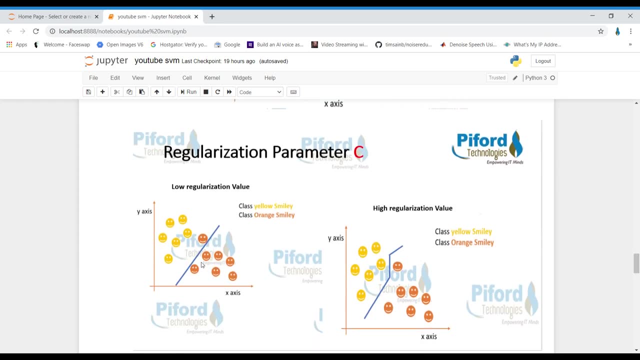 High gamma means we want to choose only the closest point to find out this. finally, hyperplane- the good hyperplane- and low value of C means there will be some accuracy. you know this classification error and with high value of C you will get more accurate classification. 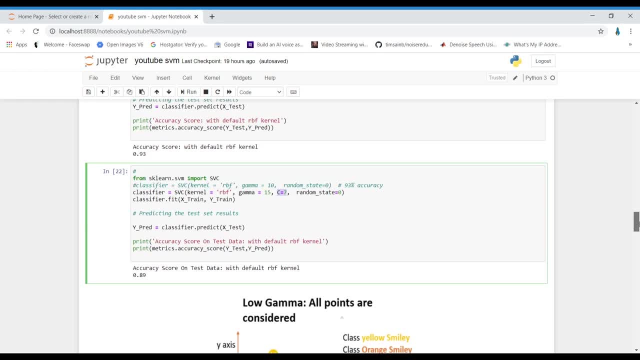 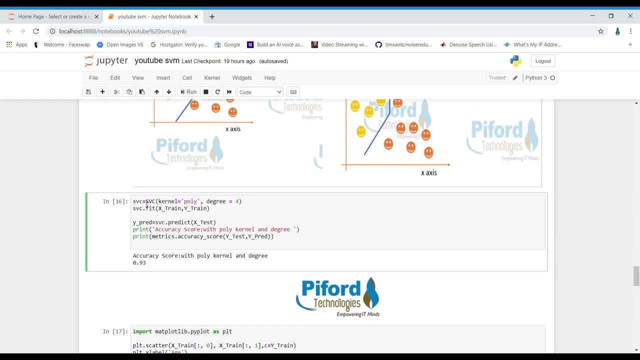 So this is what I have done here till now. Now, the next thing is: now let's use polynomial kernel. See, now I am using SVM algorithm again, but this time the kernel I am using is polynomial kernel and the degree I am giving is 4.. 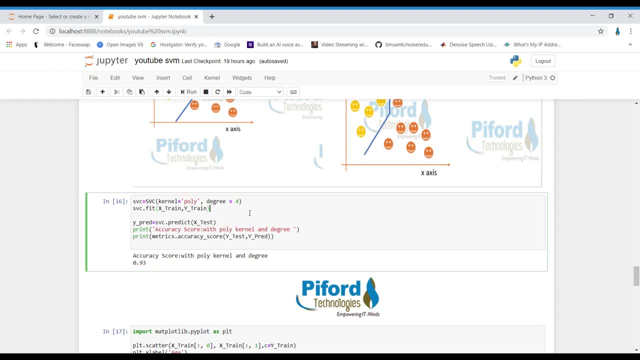 So, if you remember about polynomial regression algorithm, in polynomial regression we give different degrees to our algorithm, right? We give different degrees, we assign different degrees to our data set, So to get more good results. because polynomial regression is used to handle non-linear data, right. 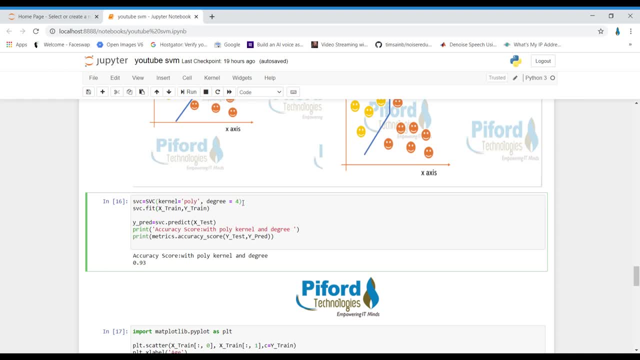 The same way, the task which polynomial regression algorithm does, same task can be performed by using kernel poly of SVC, and this degree we have to give by ourself only. So over here I am choosing degree 4 and I am training my algorithm, and then I am testing the algorithm and checking accuracy. 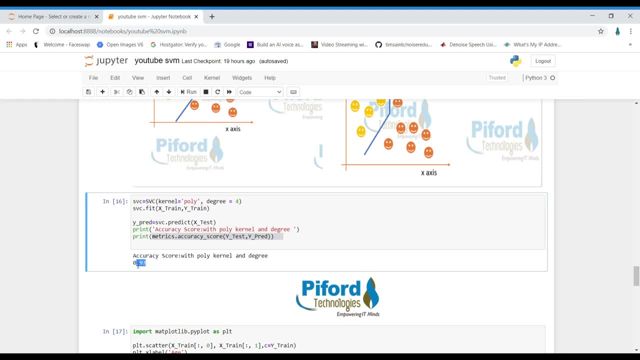 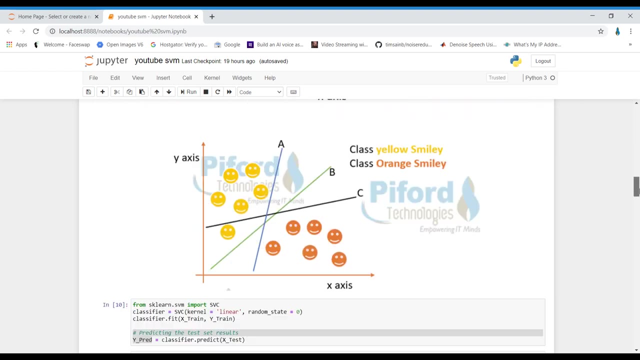 You can see that the accuracy again we are getting here is 93%. See, with RBF kernel and with this polynomial kernel we are getting accuracy 93%. but when I have used linear kernel on it you will see over here When we have used this linear kernel. 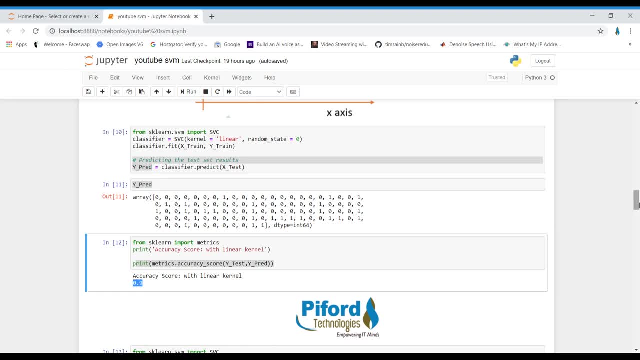 at that time I was only getting accuracy of 90%. So what we can understand from these results? that the data, the data set on which we are working upon, that data set is not a linear data. So that's why we are not getting good accuracy. 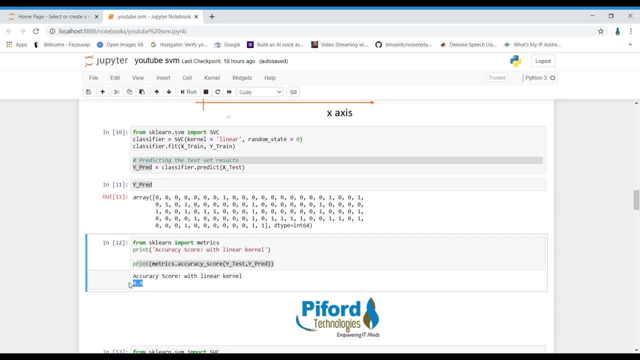 as compared to non-linear- you know- kernels. So the data set which we are using is non-linear data. So that's why we are getting better accuracy with RBF and polynomial kernel, because RBF and polynomial kernels are used to perform classification on non-linear data. 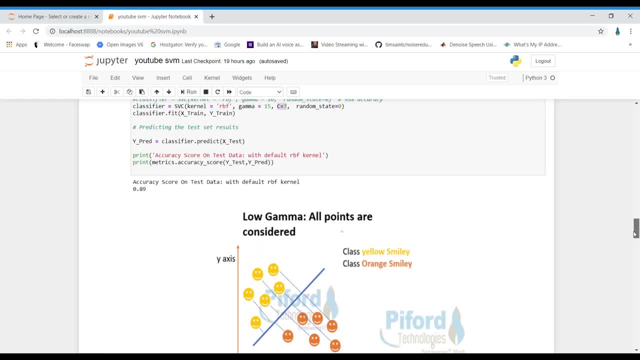 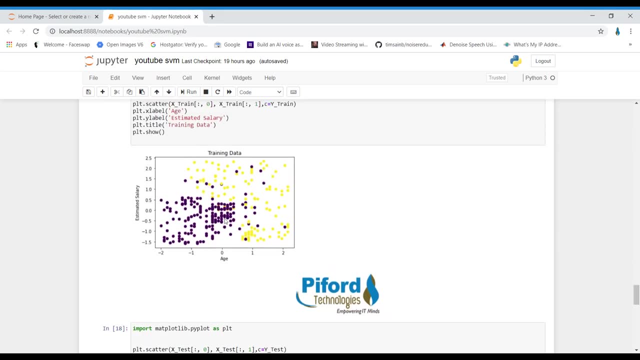 So if you want to see the data set, let me show you the data set in the form of this. So this is the training data. So over here you can see these purple points belongs to class 0 and these yellow points belongs to class 1.. 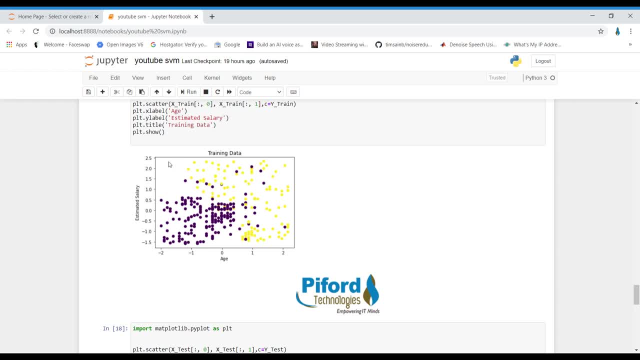 So this data is not linear? How we can say that this data is not linear? Because by just putting a straight line we cannot classify the data properly. Some of the points of this class are on this side means the data is non-linear data. 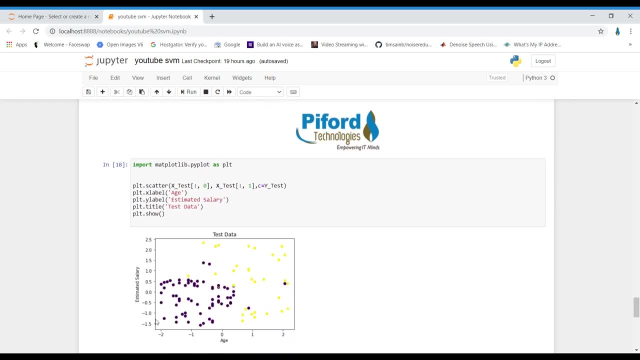 In the same way I'm plotting test data over here. In test data over here also, you can see this data is not linear, because by simply putting a line we cannot classify our data, So this data is non-linear data. So now let's draw a hyperplane. 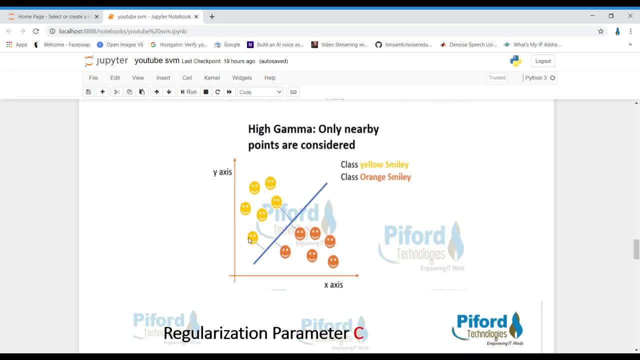 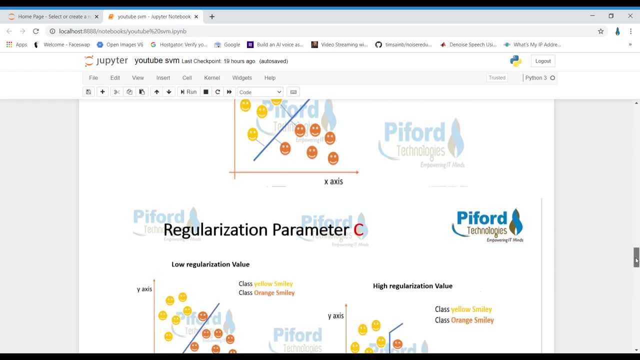 the topic which we have just discussed: the right hyperplane, How SVM classify the data By putting a right hyperplane. Let me show you how to draw that hyperplane. So that is what I'm doing over here. So this is the data. 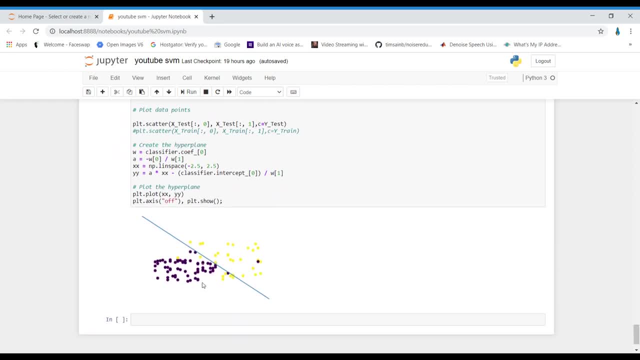 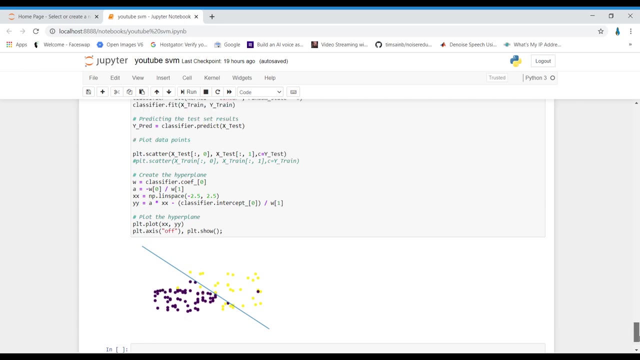 This is the data. These data points belongs to zero class and these data points- yellow data points- belongs to one class, And this is our hyperplane, right hyperplane, which is classifying our data, And this is how I have drawn this hyperplane.